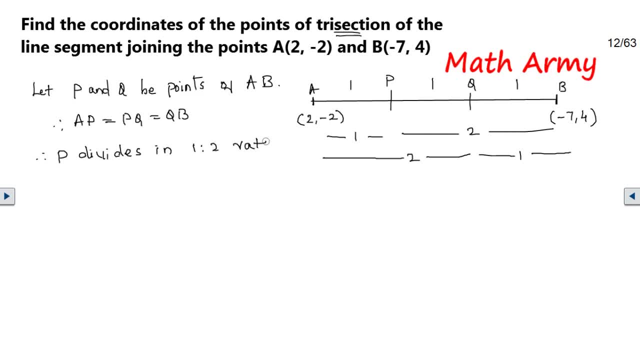 now. so what is the section formula? it is very simple: m 1 x 2 plus m 2 x 1 divided by m 1 plus m 2, right? so the same formula i am going to use. and what is m and n for me? 1 and 2 respectively. so now 1 multiplied with x 2, which is minus 7. 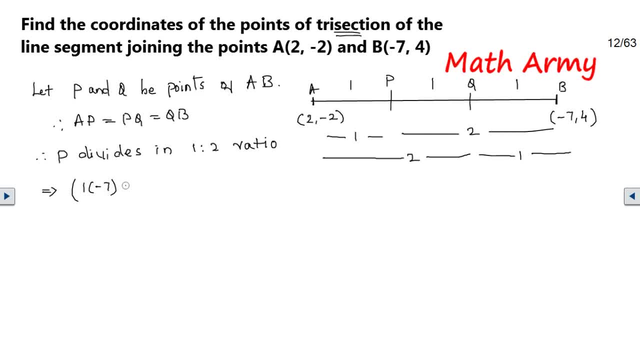 and 2 multiplied with 2 divided by 1 plus 2, which is m1 and m2. in the similar way, 1 multiplied with 4 and 2 multiplied with minus 2 divided by 1 plus 2. so if i calculate this one, i will be getting the p squared. 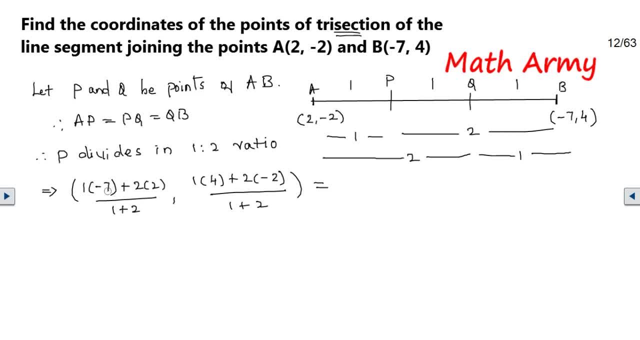 now minus 7 and 4 is going to be minus 3 and minus 3 divided by 3, because you'll be showing 7 and 4 again and plus 4 in the similar way. here it is 4 minus 4 divided by 3. minus 7 and plus 4 is going to be. 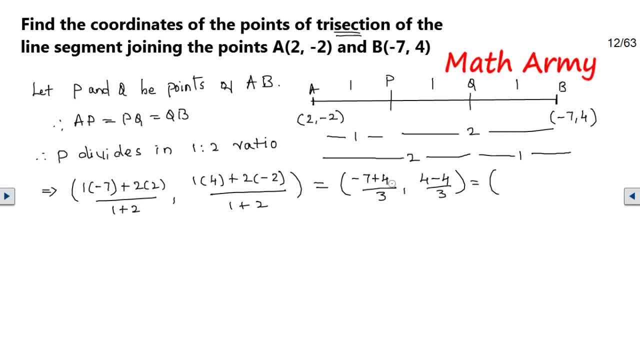 minus 3 and minus 3 divided by 3 is going to be minus 1 comma. 4 minus 4 is 0, 0 by 3 is 0, and this is the value of p. so you can write that. now let us calculate the q value. everything is. 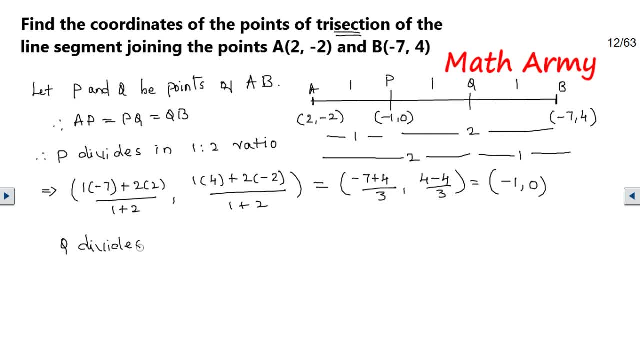 same, but only thing is the ratio: instead of 1 is to 2, for p it will be 2 is to 1 and everything. the calculation and the values are the same. now here: 2 multiplied with minus 7 and 1 multiplied with 2 divided by 2 plus 1.